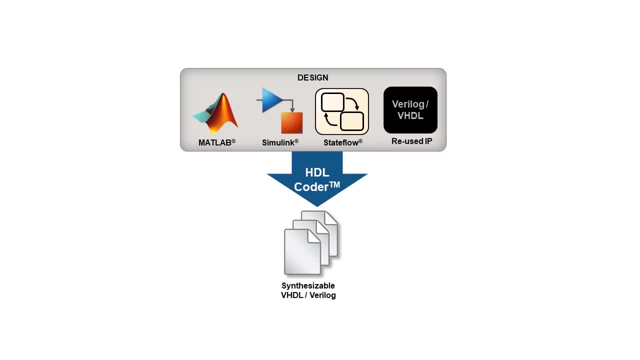 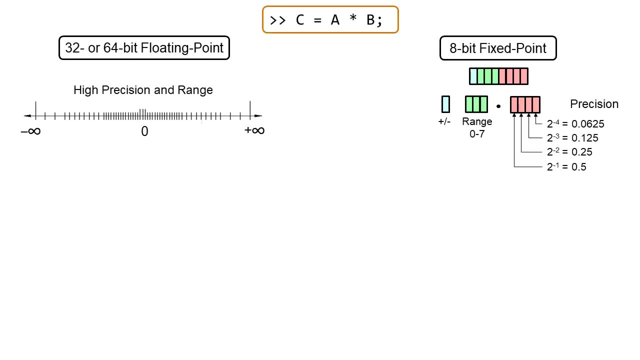 HDL Coder deploys your Simulink and MATLAB algorithms to FPGA or ASIC hardware. While most of these algorithms start off in Floating Point, quantizing to Fixpoint can greatly reduce hardware resource usage, and operations require fewer steps, But converting all your 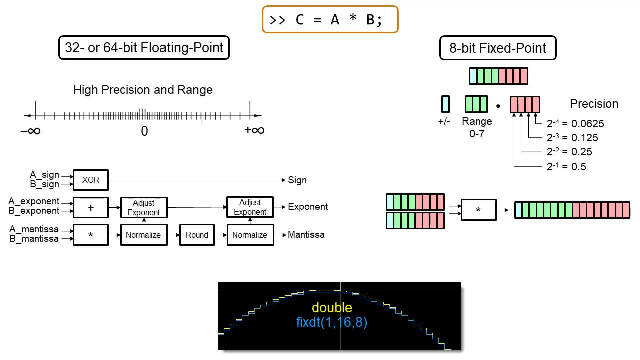 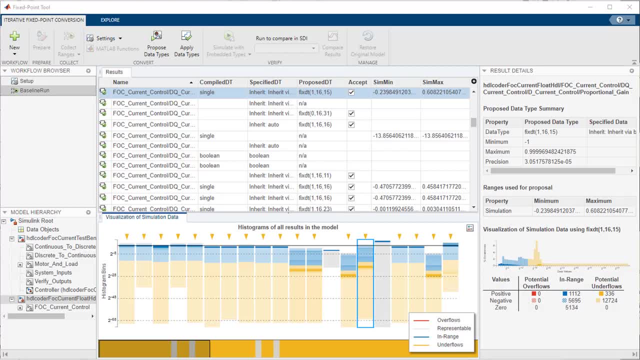 data and operations to the smallest Fixpoint word lengths, while maintaining enough accuracy, can be very time consuming and iterative. Fixpoint Designer provides guidance, automation and visual feedback to help you manage this process, But there are many designs or parts of designs that have numerical requirements that make Fixpoint conversion extremely challenging. 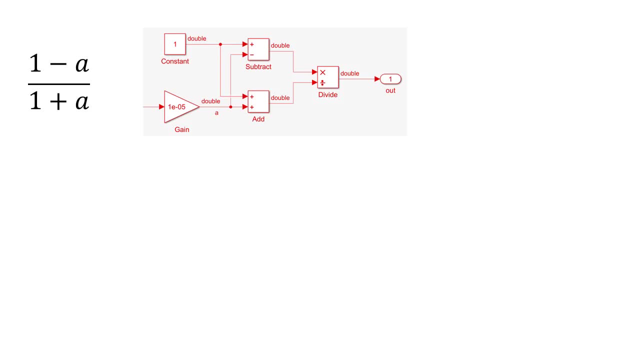 We see this a lot with motor and power control radar and certain wireless algorithms. In fact, one of our power control customers was trying to implement this simple math function as part of their design targeting an FPGA, But this function has a high dynamic range. 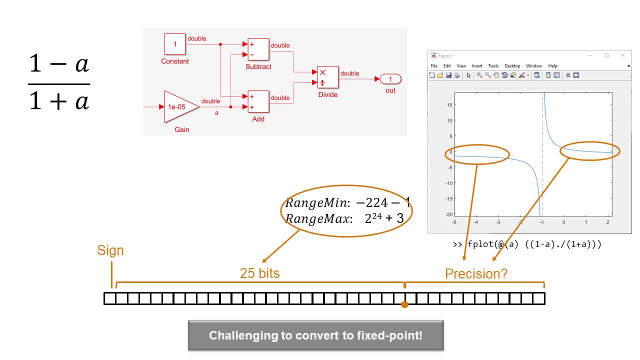 Depending on the input. sometimes the results require a lot of bits on one side of the radix point and others require a lot of bits on the other side. So it's difficult to fix a word length and radix point without throwing a lot of bits at the problem. 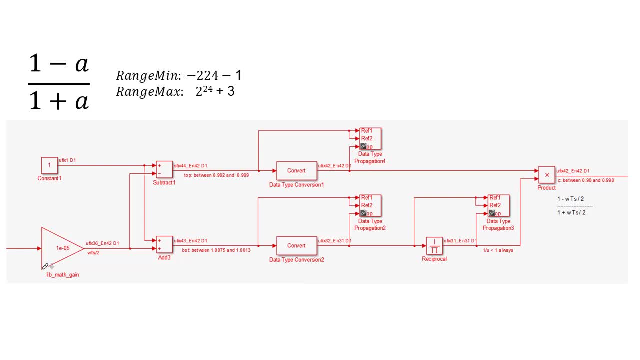 To implement this in hardware, our customer began the Fixpoint conversion process, which required some adaptations. For one, they had to break the divide operation into a reciprocal and multiplier in order to have finer control over the Fixpoint word length. And then they 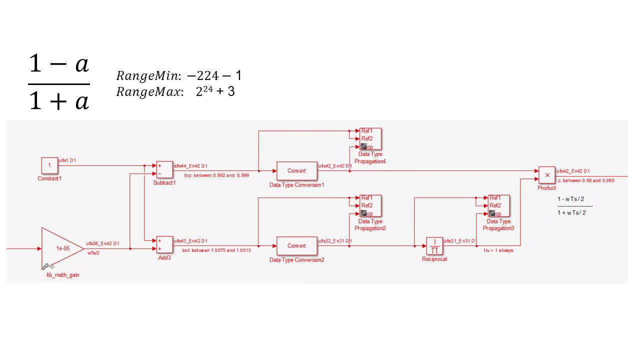 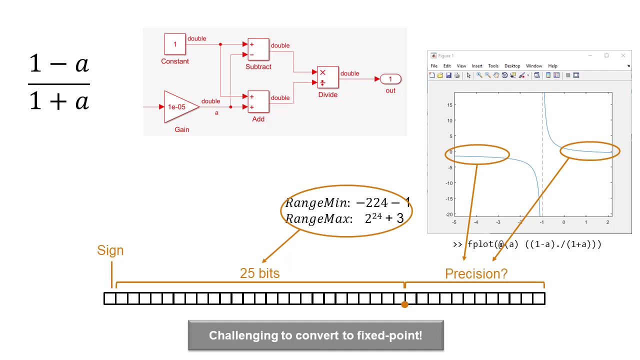 had to do a lot of work on the lookup table and the Newton-Raphson architecture for that reciprocal operation. So even for a simple math function, converting to Fixpoint is not straightforward if the math has a large dynamic range. But what if there was a way to build hardware without 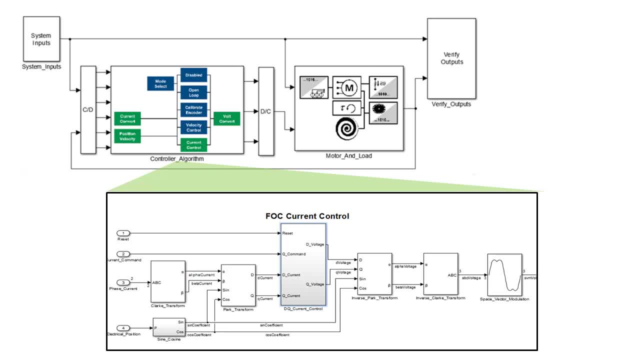 having to go through all this. In this field-oriented controller design, there are some operations, like we previously saw, that require a lot of bit length and a lot of bits at the bottom, And then there are some operations that require a lot of bit length and a lot of bits at the 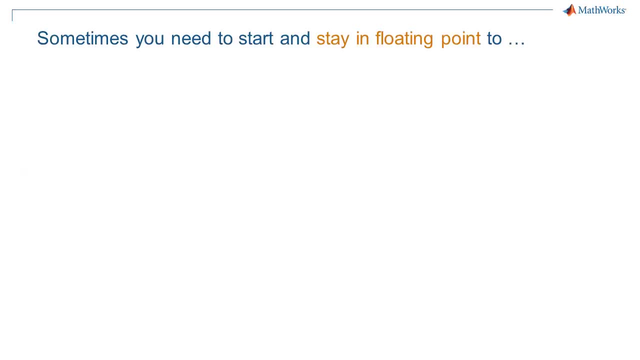 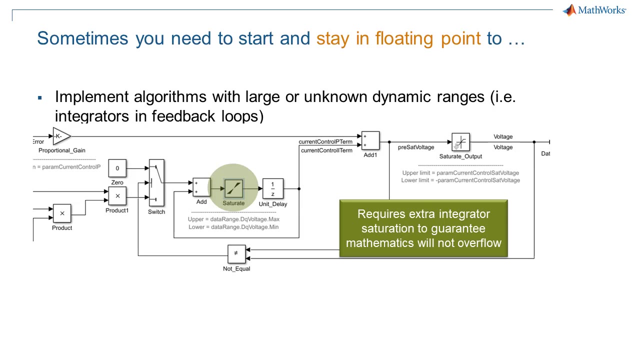 bottom, For example, algorithms with large or unknown dynamic ranges, like integrators and feedback loops, Or the saturation block here that had to be added to prevent overflow, Or operations that are difficult to design in Fixpoint, like an ATAN2 and other trigonometric functions. 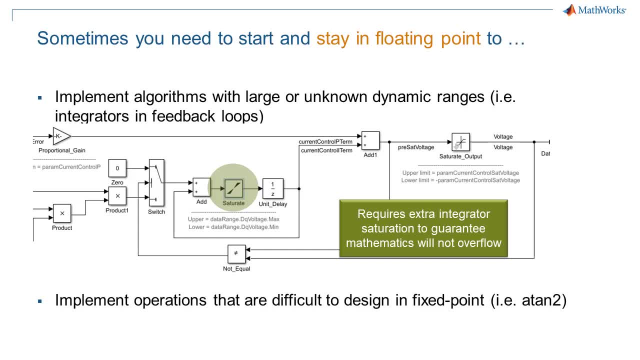 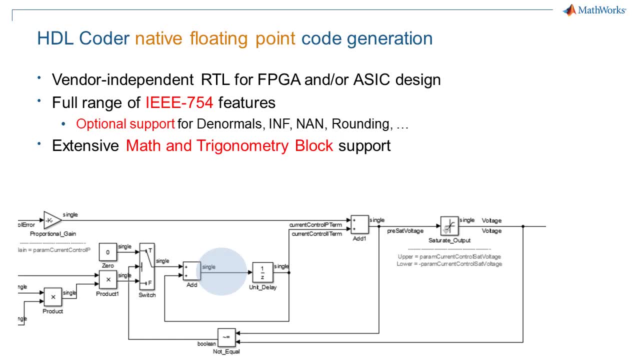 that typically are implemented in hardware as lookup tables. Now models like this can be taken directly from Floating Point to Setpoint. HDLCoder generates vendor-independent HDL from Floating Point models- double, single or half-precision. There's a wide variety of math and trigonometric functions to choose. 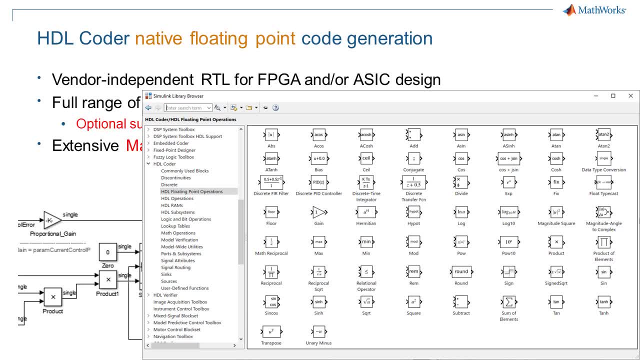 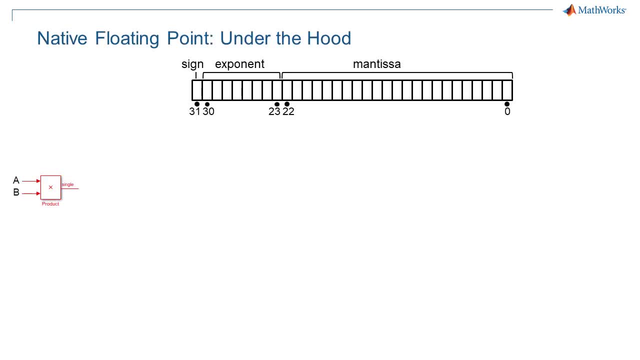 from, And the full range of IEEE 754 features is supported, including DNormal and INF-NAN. But how does HDLCoder actually implement Floating Point models in Fixpoint? Well, there are a number of ways to use HDLCoder in Fixpoint operations using fixed-resource hardware. 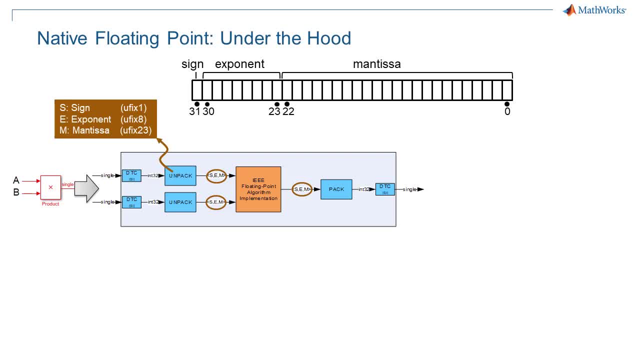 To illustrate using single precision. it starts by converting data to a 32-bit integer, then unpacking the sine, exponent and mantissa bits according to the IEEE spec. Once it has split the data into those components, it uses them to perform the arithmetic operations. 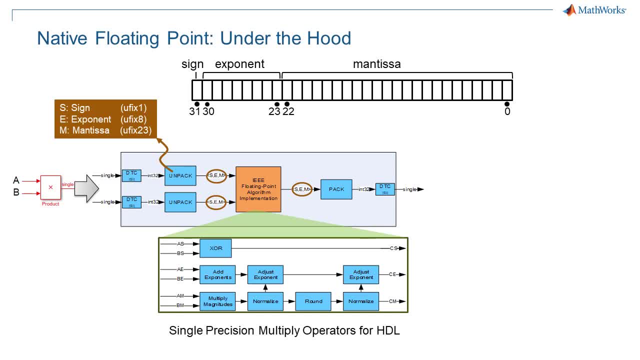 which of course are different algorithms than their Fixpoint counterparts. So in the generated HDL the inputs and outputs will be 32-bit. So in the generated HDL the inputs and outputs will be 32-bit. In the generated HDL the inputs and outputs will be 32-bit. 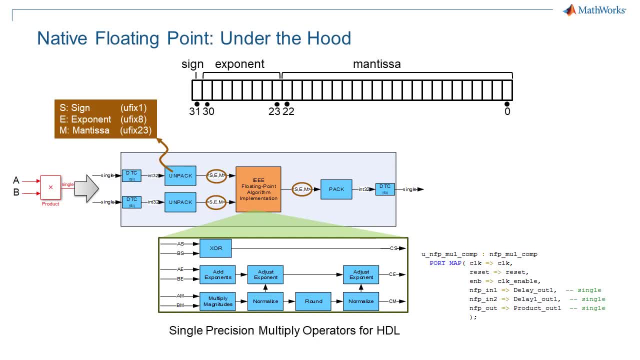 As you can see, HDLCoder only uses 32 bits and 32-bit algorithms, And Floating Point math algorithms require more steps than Fixpoint. Therefore, in cases where you can use smaller word-length Fixpoint types, your hardware will be more efficient than staying with float. 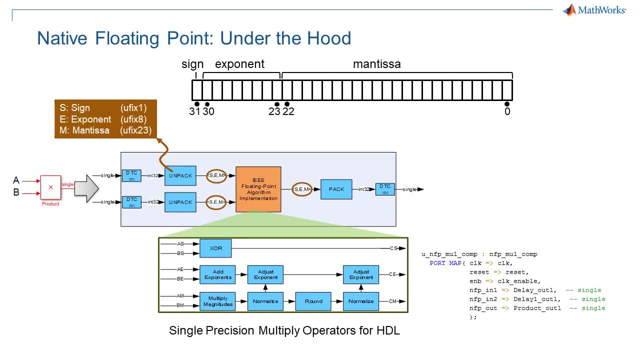 But for cases where you need a large dynamic range, it can be easier and more efficient to just stay in Floating Point. You can find the right balance for your design by mixing fixed and Floating Point operations. Let's look at an example Here in the field-oriented controller design. 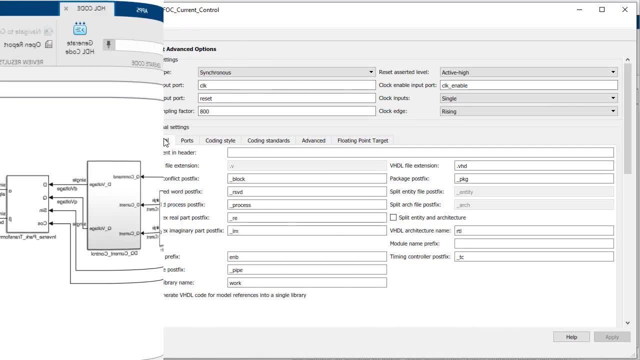 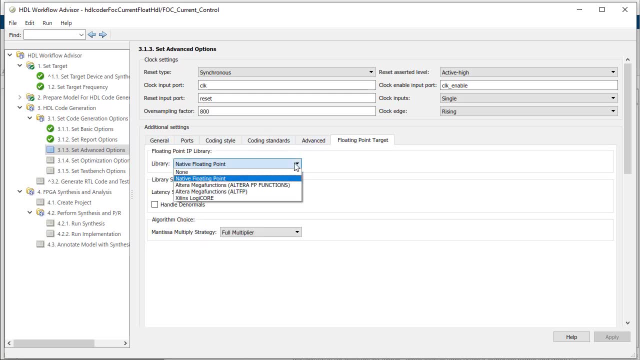 you'll notice that the data types are all single precision floating point. To generate native floating point HDL, go to the floating point target setting and choose the target. You can map to FPGA vendor macro libraries but you won't be able to see or trace into them. 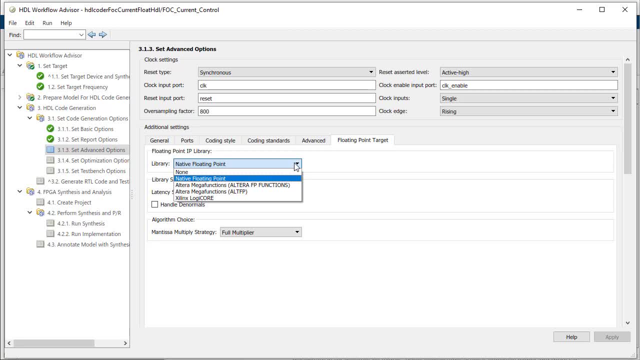 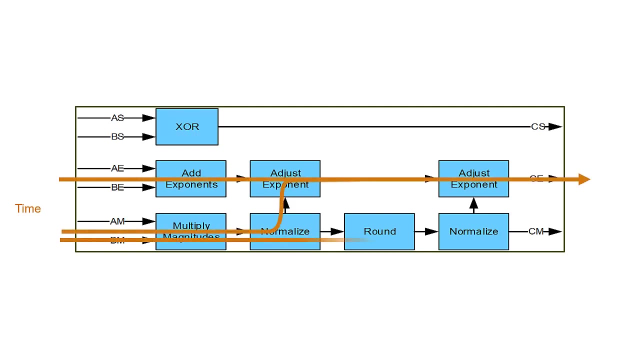 Native floating point will generate target-independent code that's completely readable and traceable. There are some customization options here. Let's focus on latency. Remember floating point. math has some extra steps and this extra logic takes time for data to propagate through it. 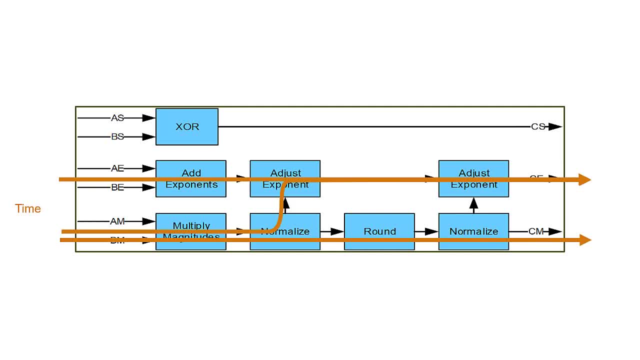 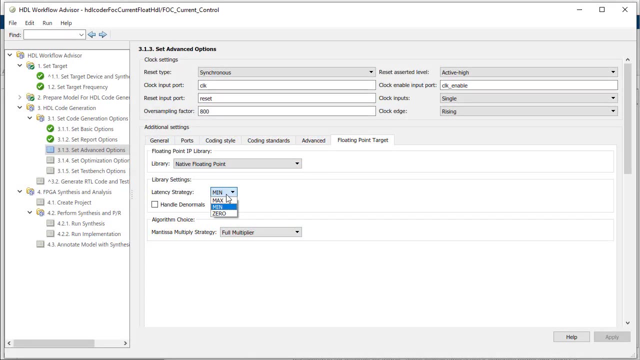 If you were manually writing RTL, you would shorten these paths by inserting registers. It makes it easier to synchronize signals from converging paths, and shorter paths mean you can run at a faster clock rate. HDL Coder provides some options here. For instance, you could try zero latency. 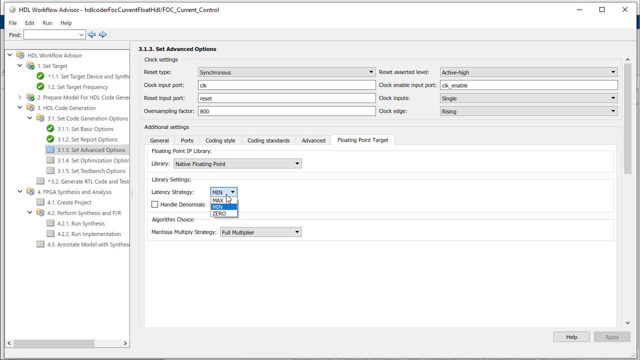 in which case you could run at a faster clock rate. In this case, you would have some really long paths forcing you to use a slow clock rate. If you try one of the other choices, you have to set the oversampling factor. 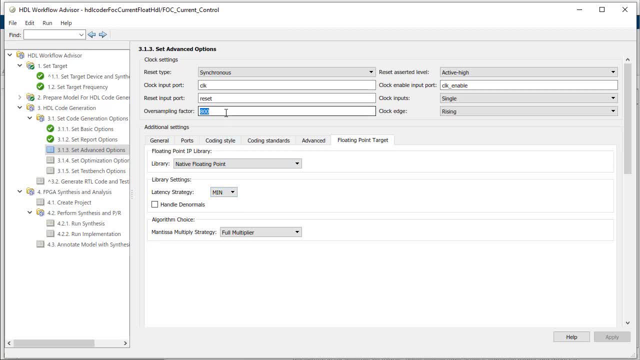 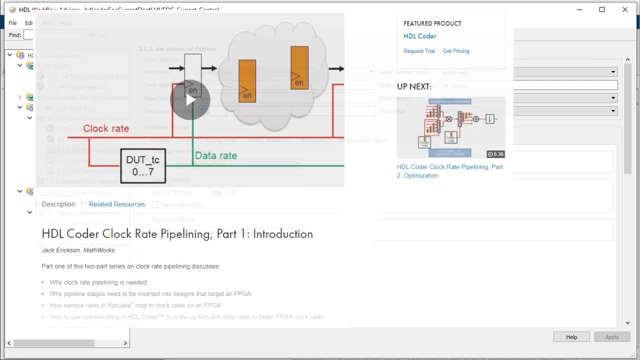 because you don't want to insert registers at the design sample rate. That would increase latency through the design. For more on this, I encourage you to check out this video. For this design, the sampling rate for the inputs and outputs is 20 kilohertz. 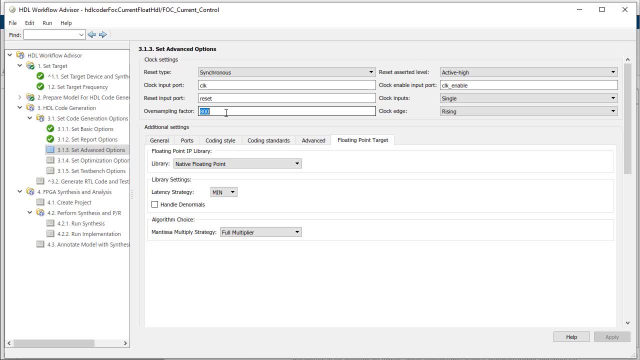 By setting an oversampling factor of 800, that assumes we can run the FPGA. You can run the FPGA at 40 megahertz and any inserted registers will also run at that clock rate. The default setting here is min latency, which provides a nice balance. 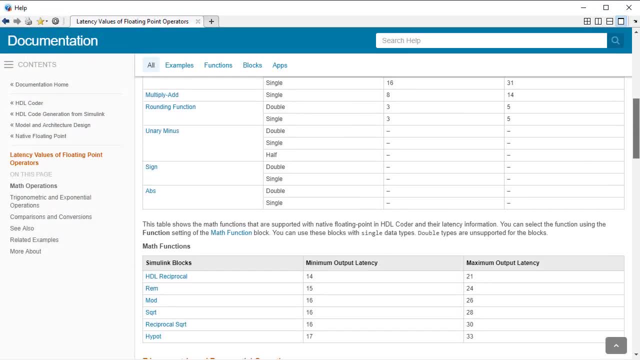 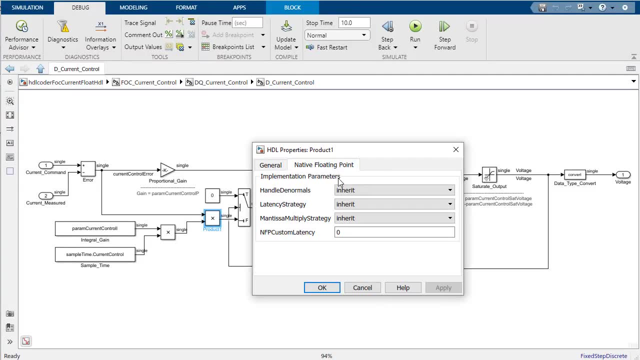 If you want to see the min and max for each operator, they're all listed here in the documentation. And if you want even more control, you have the ability to set this for individual blocks and you can even specify a custom latency value. 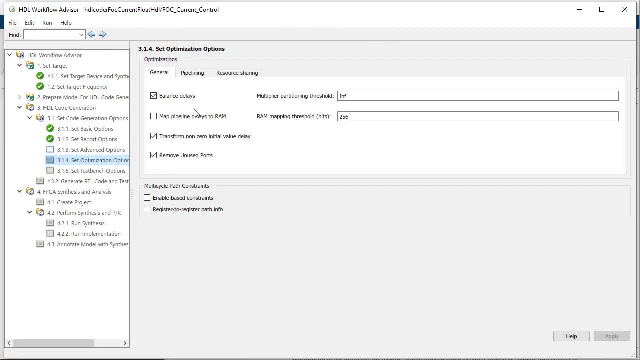 Moving to the optimization settings and looking at the resource sharing tab, there is an option there to share floating point operators. It's on by default because all optimizations are supported as part of native floating point. The first example here is resource sharing. 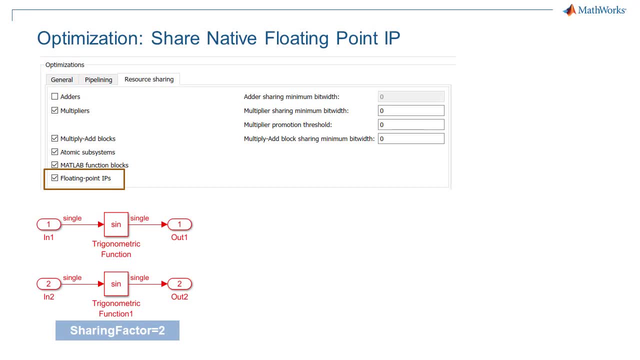 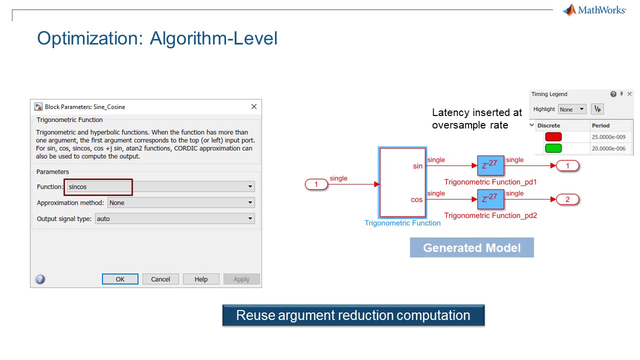 This is a simple example of two floating point sign operations And with resource sharing enabled they can be time multiplexed so one fixed resource can be shared for both operations. Even more powerful is algorithmic level sharing. Take the case of a sine and cosine operation. 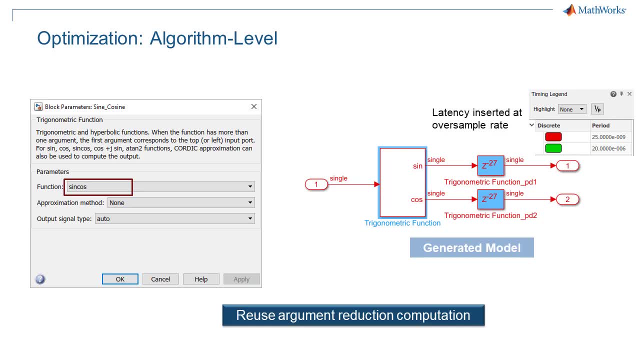 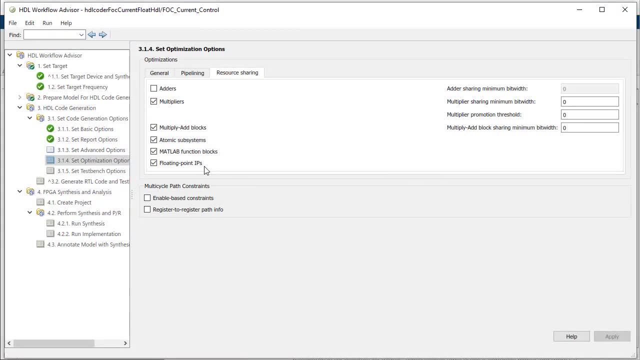 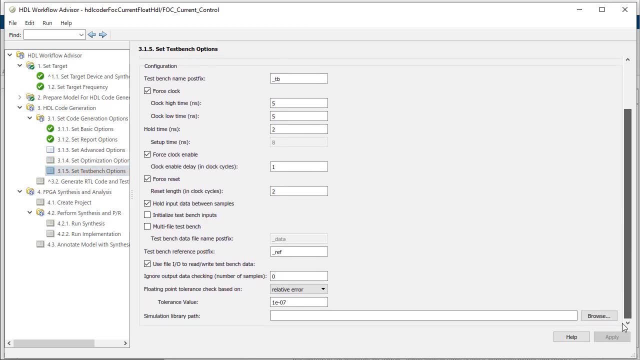 The underlying argument reduction computation can be reused between both. Designing the hardware at the algorithm level provides more opportunities for high impact optimizations like this, And if you're going to generate a test bench as part of the HDL Coder run, there is an option to specify error checking. 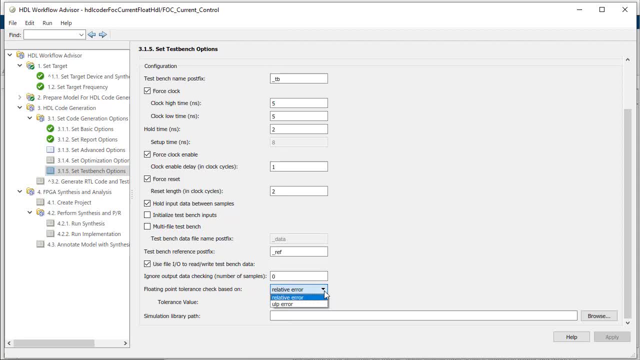 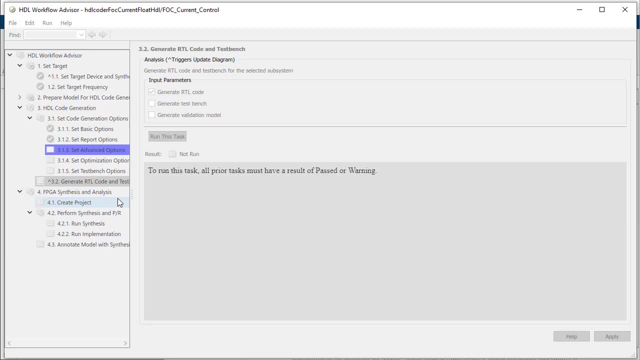 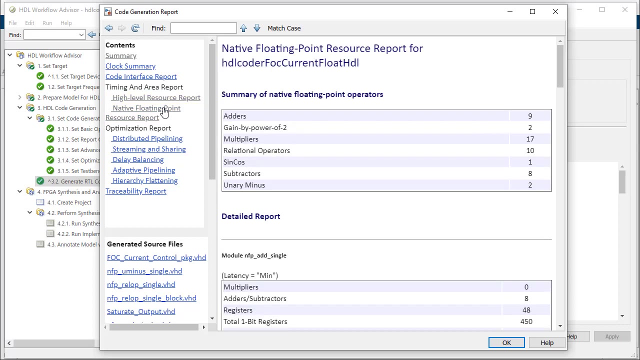 to use relative units in last place. So the test bench will ignore small bit errors in the least significant bit of the man test. The code generation report will have a native floating point section of the resource usage report which shows the resources specifically used for floating point operations. 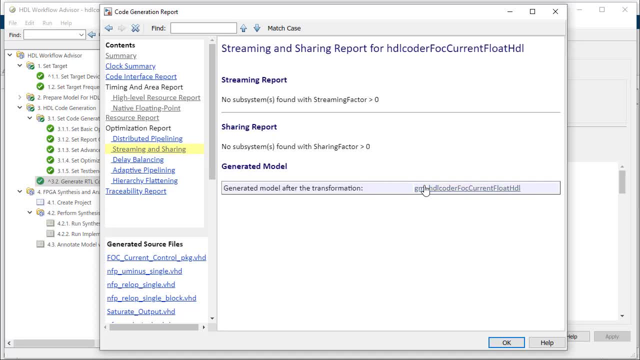 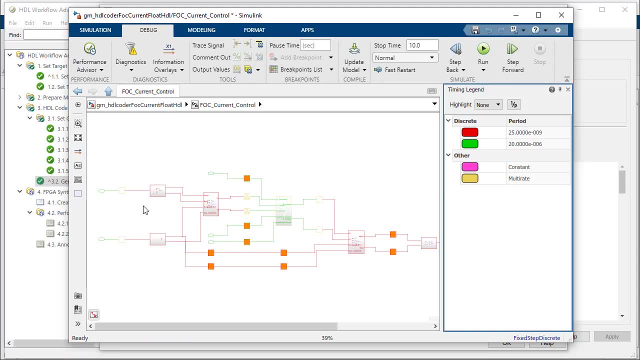 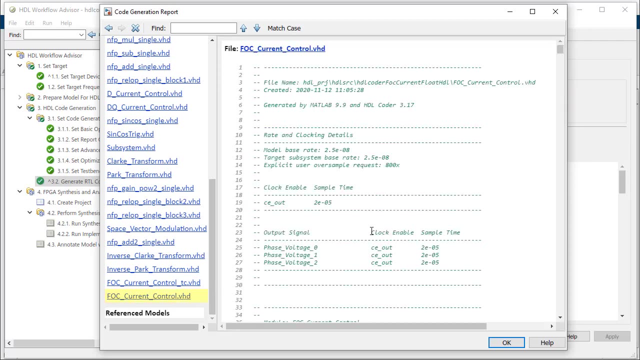 As expected, there's some overhead for using floating point operations because they require more steps In the generated model that HDL Coder produces. visualizing the sample rates shows where the 800x over sampling was applied. Looking into the code, the inputs and outputs. 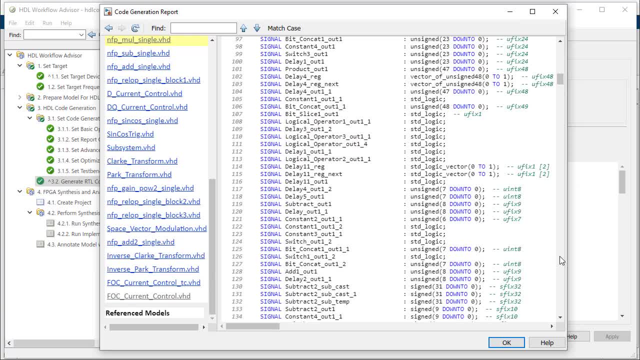 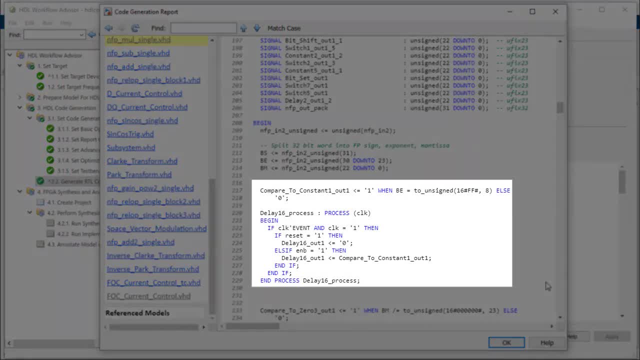 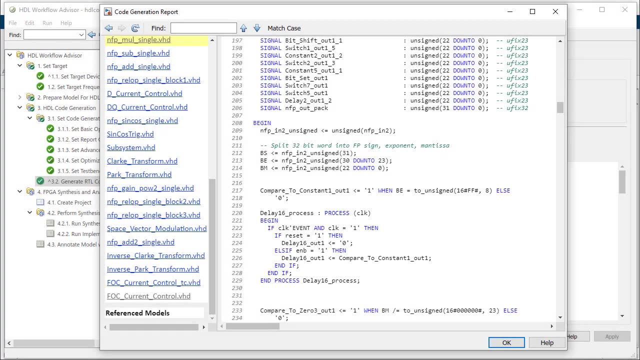 are 32 bits, as expected, And those signals get split into the sine, exponent and mantissa components. And these delay signals are pipeline registers that were added to shorten the paths through the extra steps in the floating point calculations. Now, if I want to reduce resource usage, 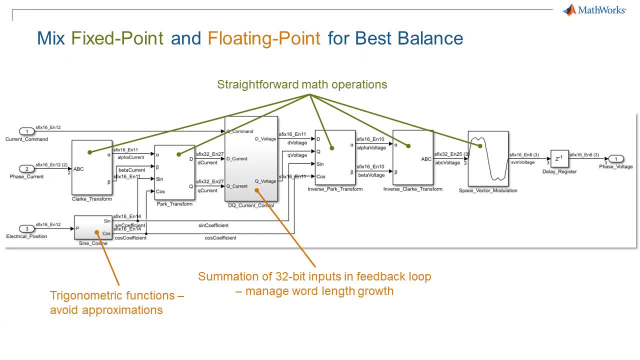 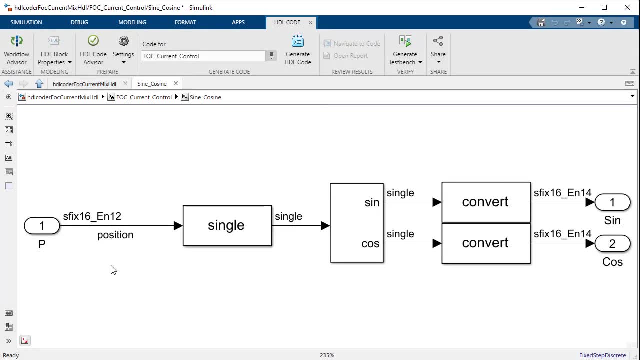 I can combine fixed and floating point in the same design. Here I've converted the same design to mostly 16-bit fixed point using Fixed Point Designer, But I've isolated and used floating point for the sine cosine operation, whereas in a pure fixed point. 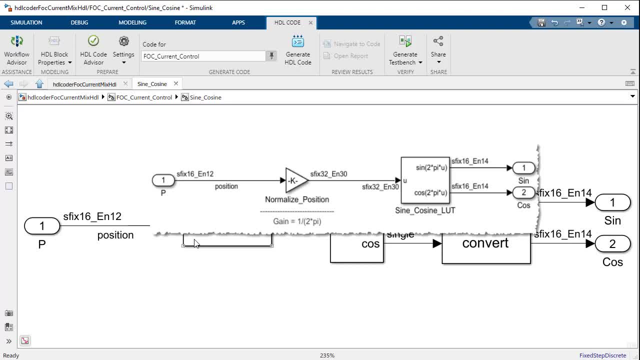 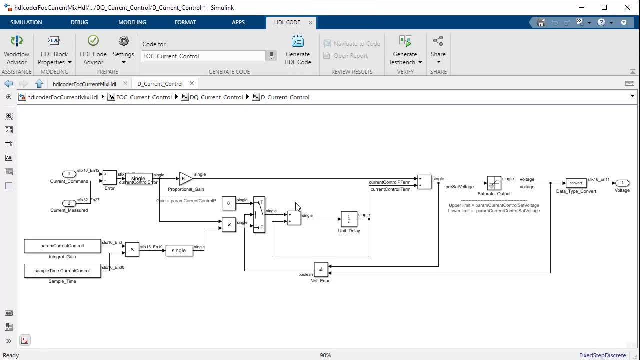 version, I had to create a lookup table for the sine cosine and use a multiplier on the input to normalize it, And the same for the feedback loop in the current control blocks, because small errors could become really magnified. Note that using floating point also. 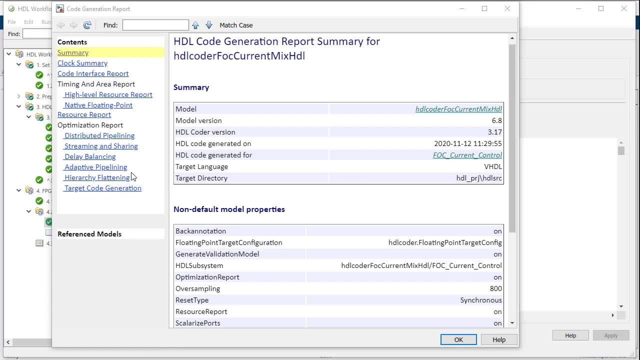 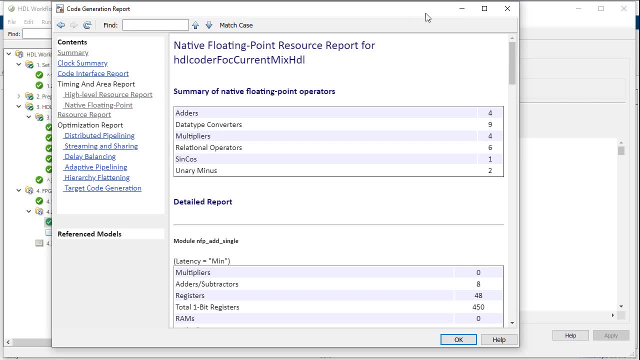 allowed me to remove the saturation logic After HDL Coder, The code generation, the improvement in resource usage is pretty clear And I had set a 50 megahertz target frequency to provide some margin over the real target of 40 megahertz. 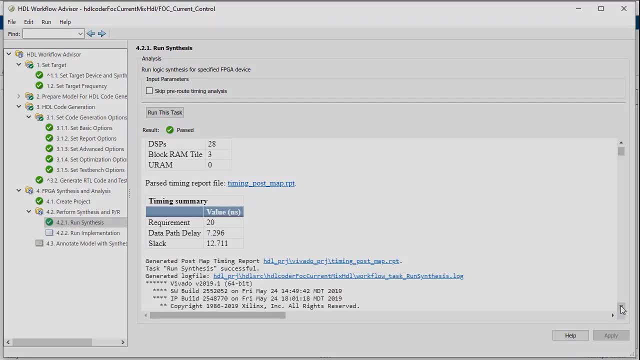 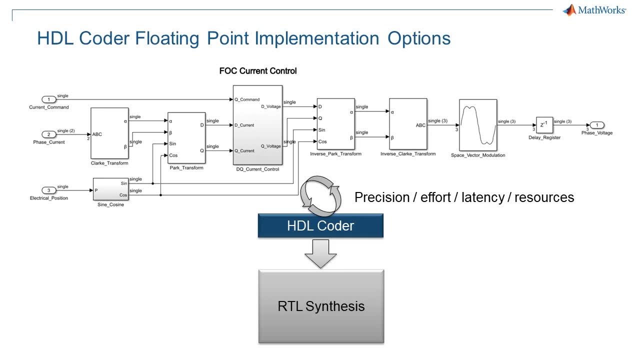 But after this is done, running synthesis it shows that there is plenty of margin And it's nice that I could iterate with an HDL Coder to get the right balance of resource usage versus precision before running all the way through synthesis. So with HDL Coder you have a few options.